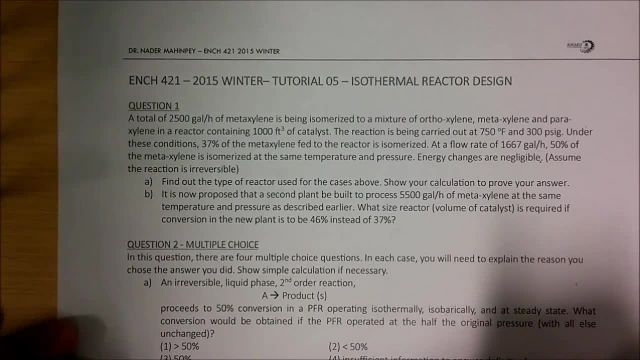 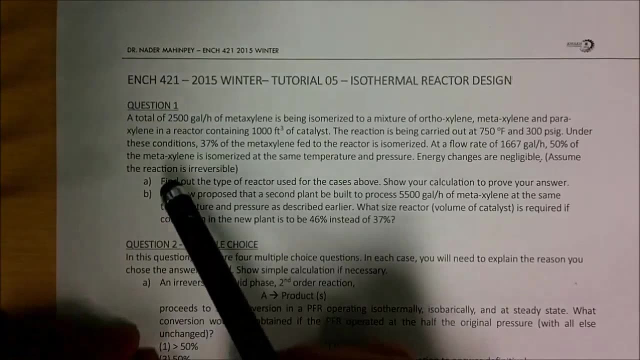 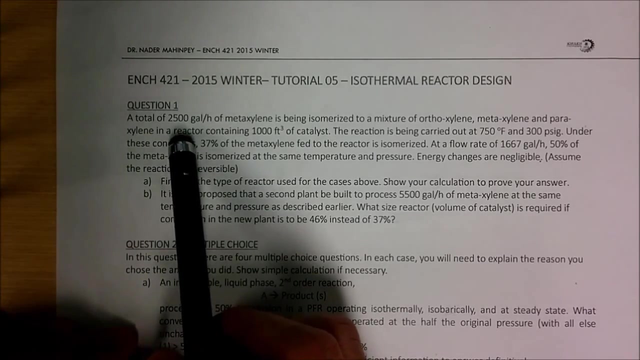 number two, we try to analyze a couple of questions related to isothermal reactor design. Let's start with question number one. In this question we're going to have a volumetric flow rate about 2,500 gallons per hour of metasyllane and it's being isomerized to 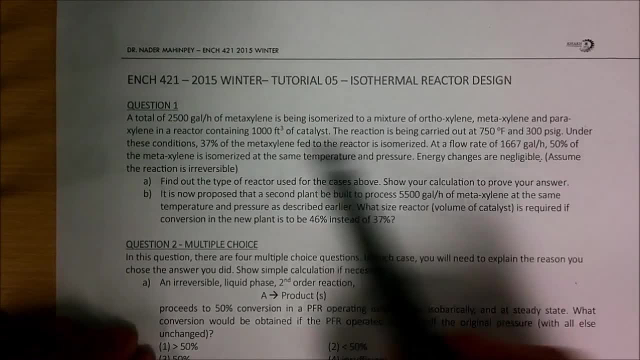 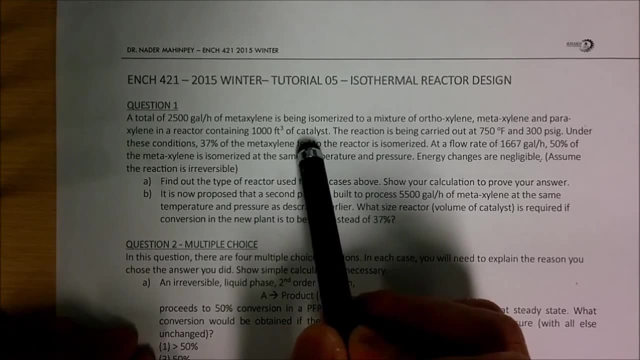 a mixture of orthosilane, metasyllane and parasyllane, And we also have the information that the reactor has about 1,000 feet cubic of catalyst. And then we have information of temperature and pressure, which is 750 degrees Fahrenheit. 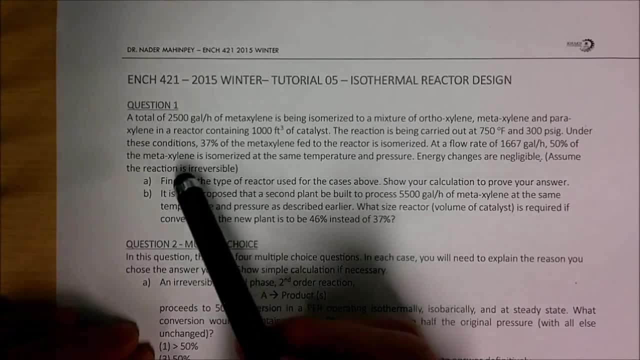 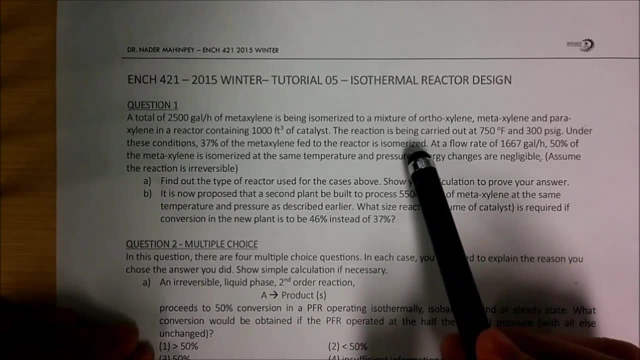 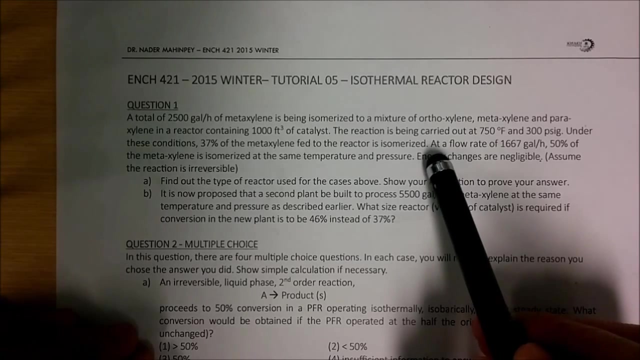 and 300 PSIG And under this condition we basically have 30% of the metasyllane fed to the reactor is isomerized, which is basically the conversion is about 37%. And then we have another information: if we run the reactor at different flow rates, we're 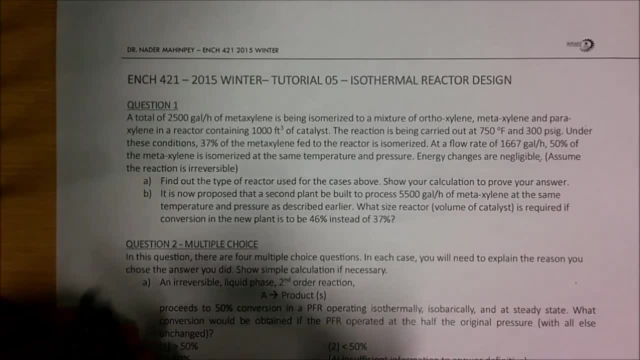 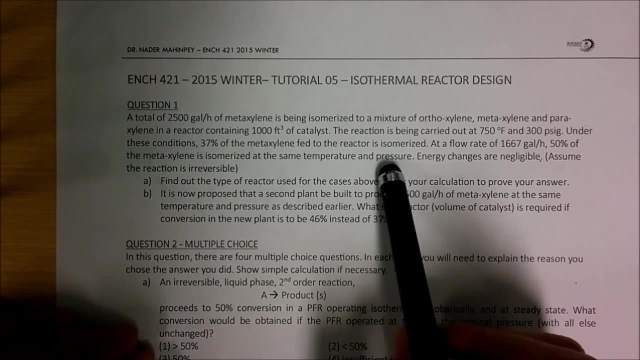 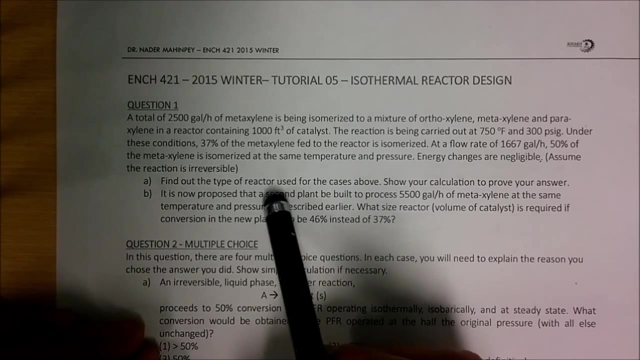 gonna have a conversion about 1.667 gallons per hour. we're gonna have a conversion about 50%, which is higher at the same temperature and same pressure. So the question is for part A, we need to find out the type of reactor use and we need 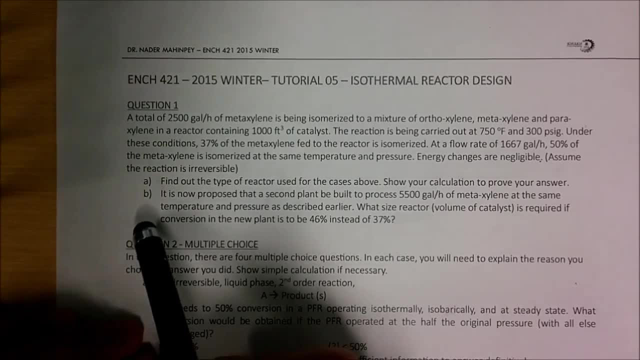 to show the calculation to prove the answer, And then, in part B, if we need to build a second plant that's bigger than this, Venom Hunters and we already have a bunch of easily focused young men who like to build bigger plants For this 44,000. Alors, we will talk a little bit about the structure and structure and we're going to talk about all the details in vivid and complex questions that you might ask us about this year: gender, when we work more and more into the technical questions for the Lipo de Mon该, Northeast and for programs related to specific issues or resources. But if you would just pause and go ahead and read the fullum american history, So as a 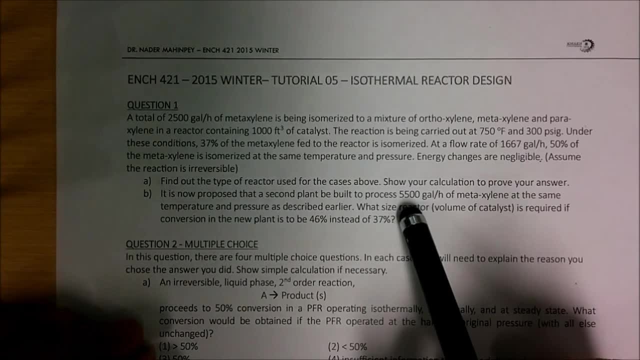 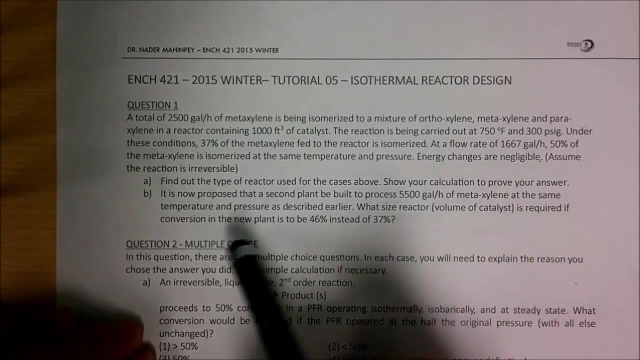 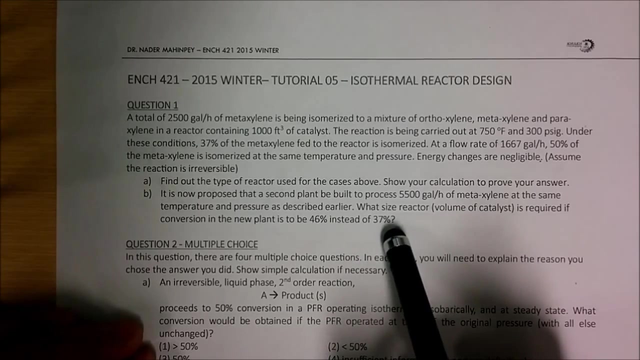 using volumetric flow rate of about 5,500 gallon per hour, the same temperature and the same pressure. now we need to calculate what's gonna be the size of reactor, based on volume of catalyst required to have a conversion. in the new plane it's about 46% instead of 37% in the previous. 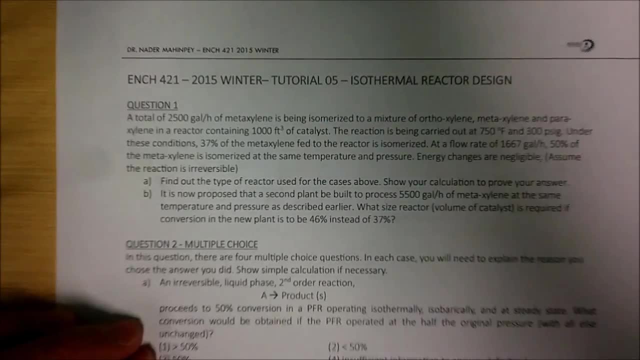 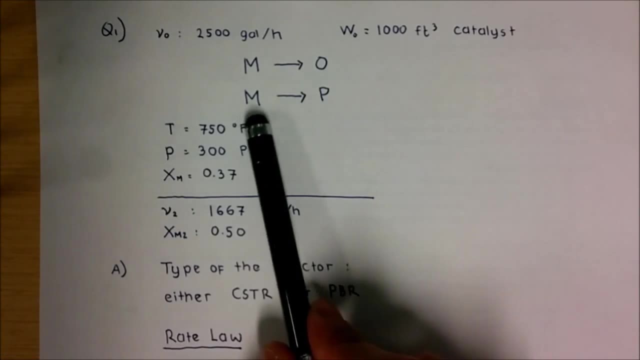 condition. in order to solve the problem, we need to list all the information that we have: volumetric, the two type of the reaction, the volume of catalyst and also the first condition, which is volumetric flow rate about 2,500, and the second condition, it's about 1667 gallon per. 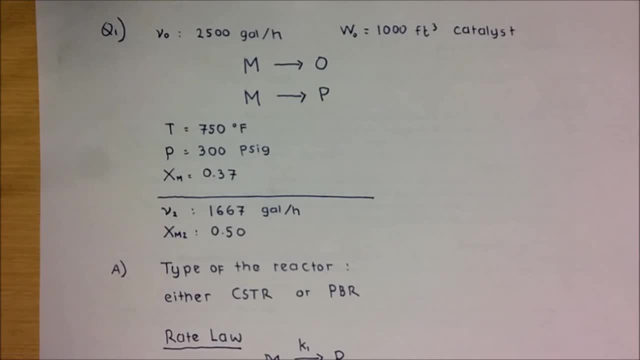 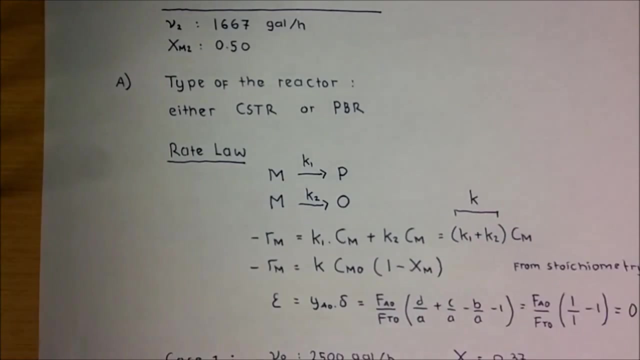 hour, with the conversion about 50%. so, in order to find out the type of the reactor, since we know that this is flow reactor, so it's going to be either CSTR with catalyst or a PBR with catalysts, and then based on the rate, 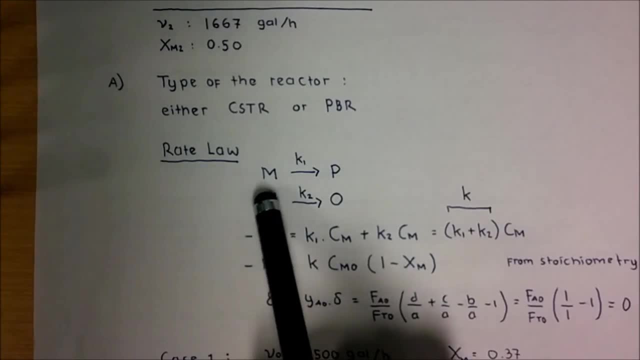 law. we can write down, for example: meta-silane goes to para-silane, we're gonna have rate constant k1, and then from a meta-silane to ortho-silane, we're gonna have rate constant and rate constant K1, and then for meta-silane to ortho silane. 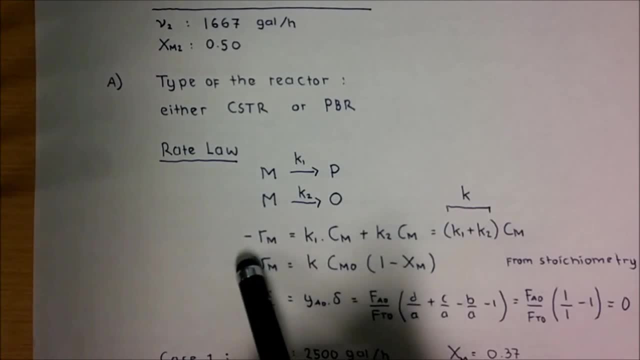 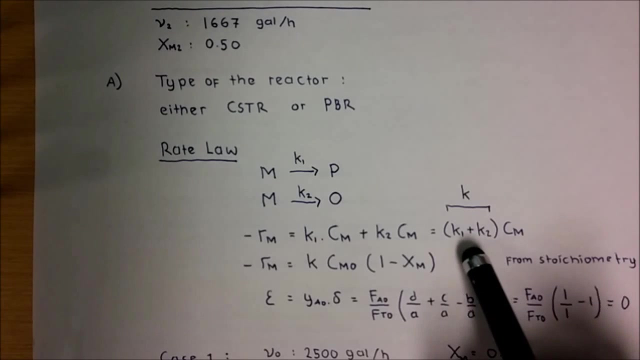 gonna have k2 as a rate constant. so if we write down the rate law for both reaction we're gonna have k1 times concentration of m plus k2 multiplied by concentration of m, and then if we combine the rate constant we can just have k multiplied by cm and from stoichiometry we can break it down. 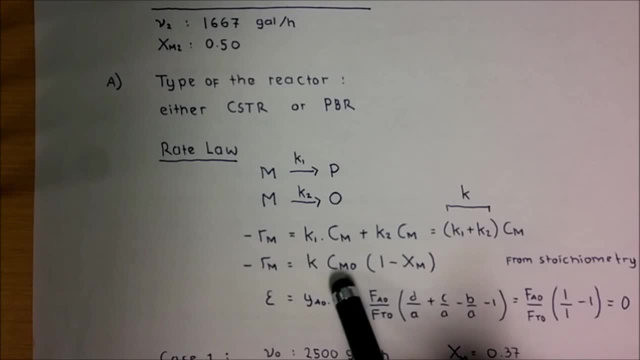 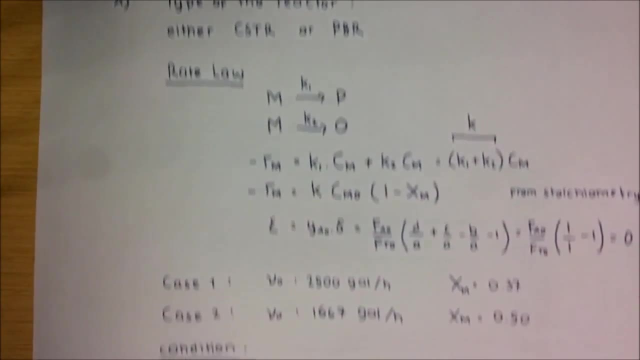 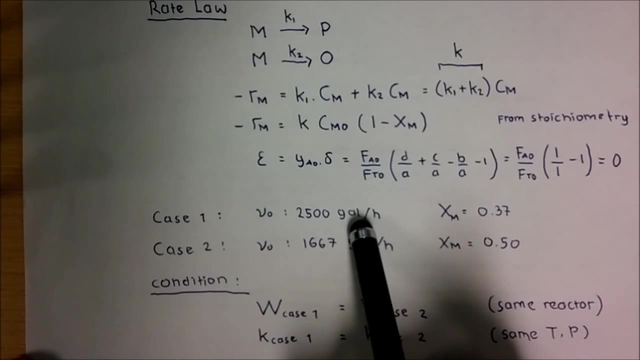 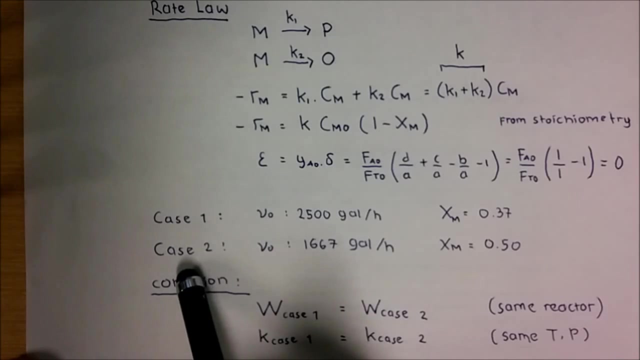 the rate law of rm is going to be k times cm, naught 1 minus the conversion. so in case 1 we're going to have a volumetric flow rate about 2500 gallon per hour and the conversion is about 37 percent. and then in case 2 we're going to have volumetric flow rate. 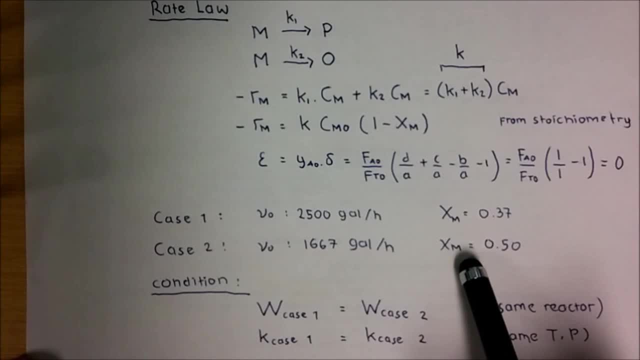 about 166 percent, and then, in case 2, we're going to have volumetric flow rate about 166, seven gallon per hour, with the conversion about 50 percent. so in order to find the reactor, we need to find the condition, since this is the same reactor that we use. what it means that? 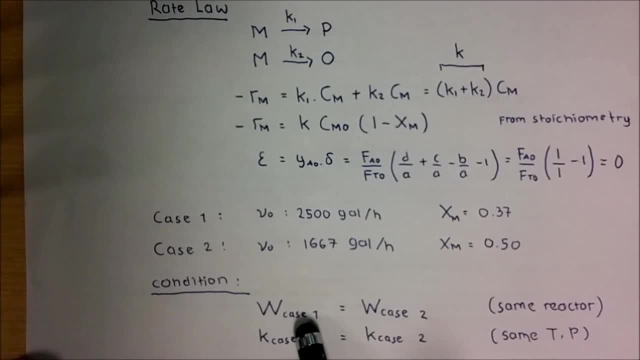 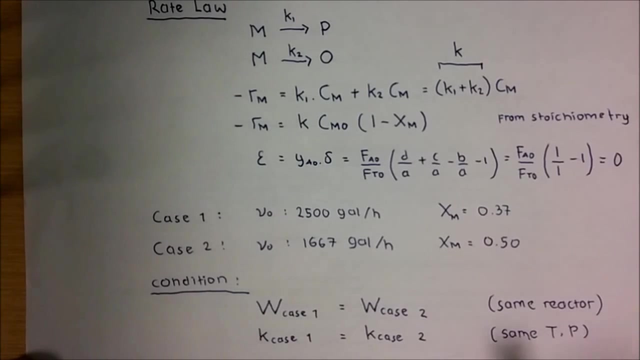 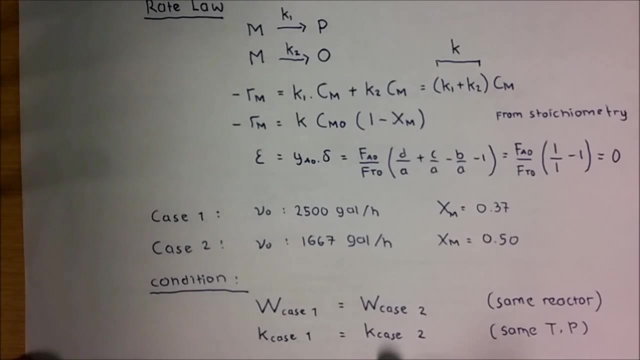 the volume of the catalyst at case one should be the same with the volume of catalyst in the case two, and we also know that since the both reaction has been done at the same temperature and pressure, then the rate constant for k, which is k at the case one, it's going to be the same with the rate constant at case two. 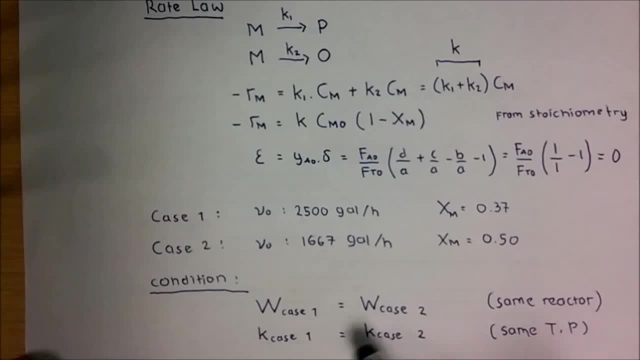 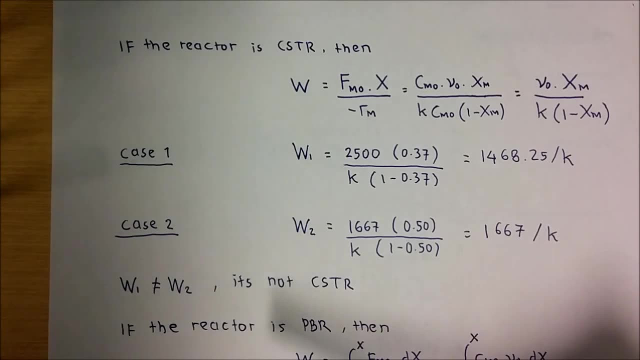 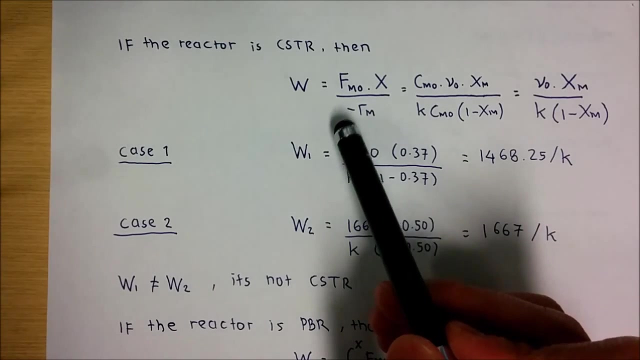 so if we multiply these two we should have the same number. so now we need to find out whether it's cstr or pbr. so we assume if the reactor is cstr, then we're going to calculate w, which is based on the mole balance equation. it's going to be f m naught multiplied by x. 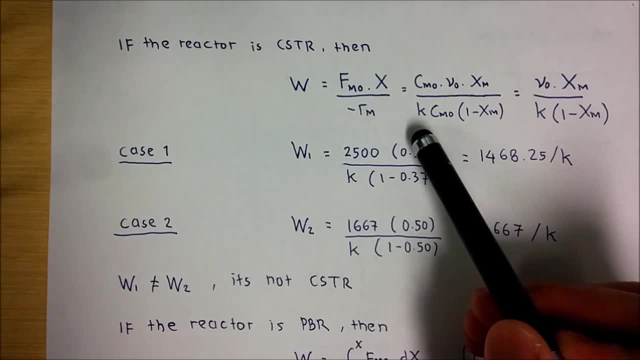 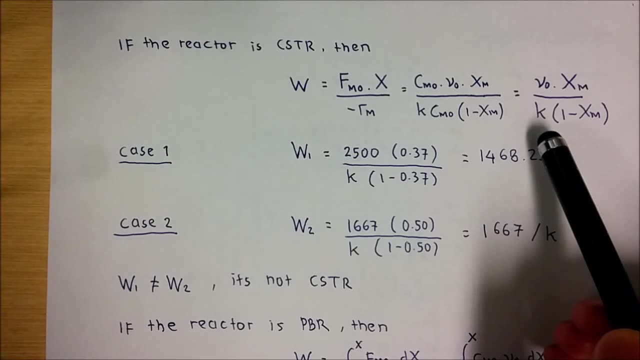 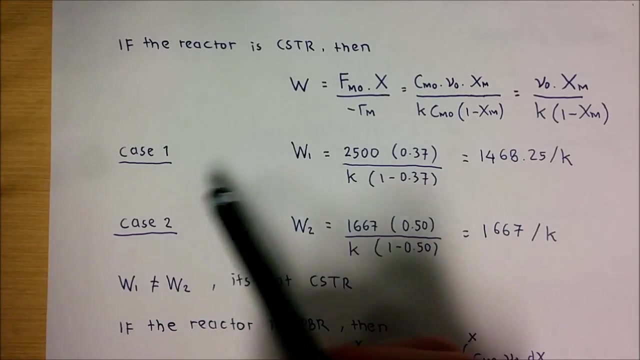 over the rate law and if we break it down we're going to have at the end the volumetric flow rate multiplied by the conversion over k, multiplied by 1 minus the conversion. so if we plug in the net, so if we plug in the number for case one, the volume of catalyst is going to be 2500. 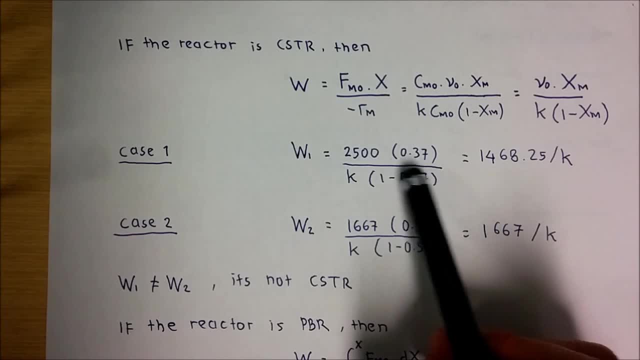 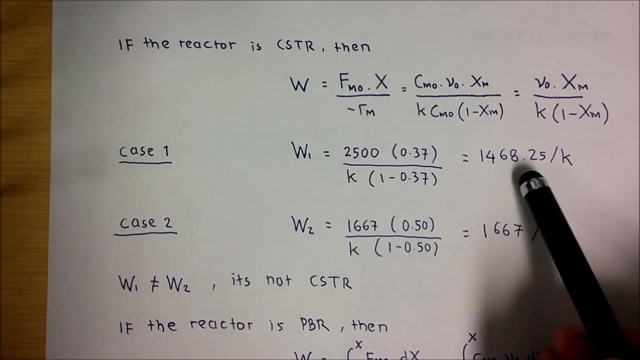 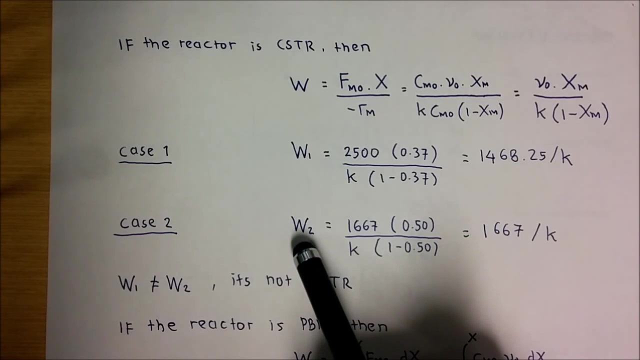 which is the volumetric flow rate. multiplied by the conversion- 37 percent over k, we don't know yet- and then multiplied by 1 minus 0.37, it's going to be equal to 1468.25 over k. and then, in case two, if we multiply, we calculate the w, we're going to have 1667. 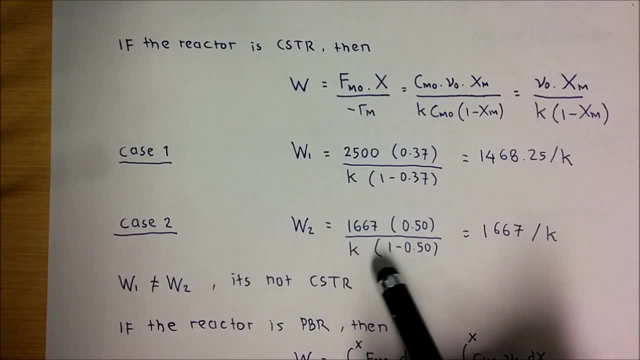 multiplied by 50- conversion over k- multiplied by 1 minus 0.5, we're gonna have about 1667 over k. so based on this calculation, we can see that w1 and w2 has this different number. so what it means? that the reactor is not cstr. 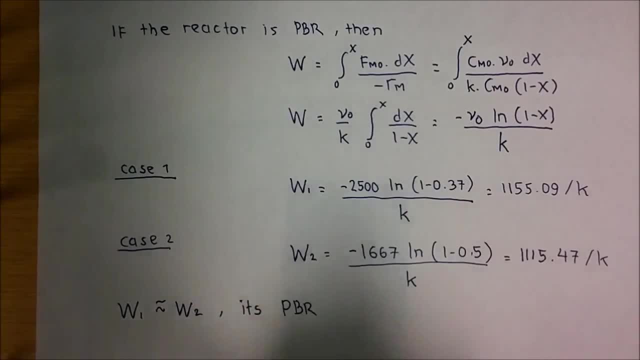 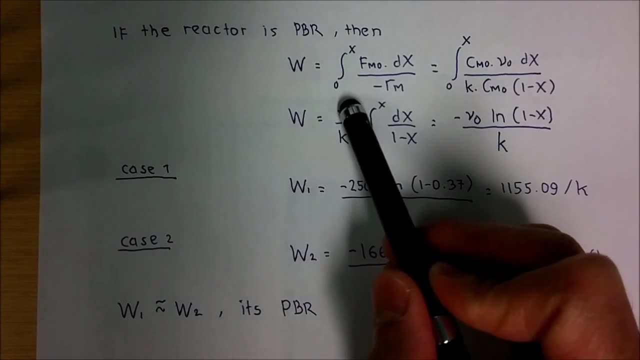 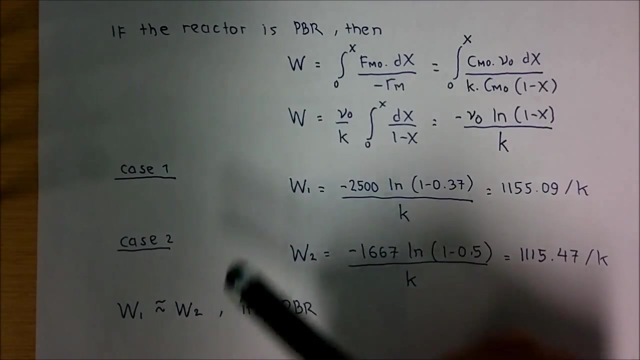 so now we try to calculate: if the reactor is pbr, then w based on the mole balance is going to be equal to the integration of fm naught multiplied by dx over rate law, from 0 to x. and then if we integrate that one based on the rate law, 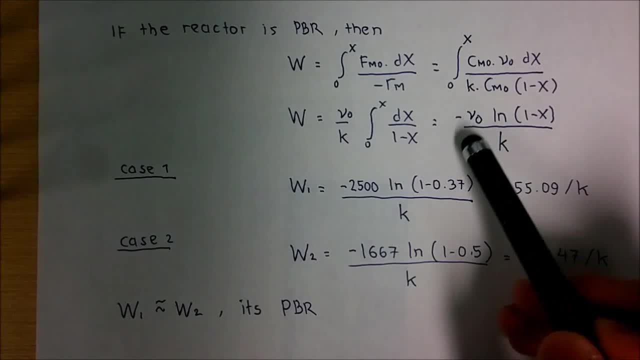 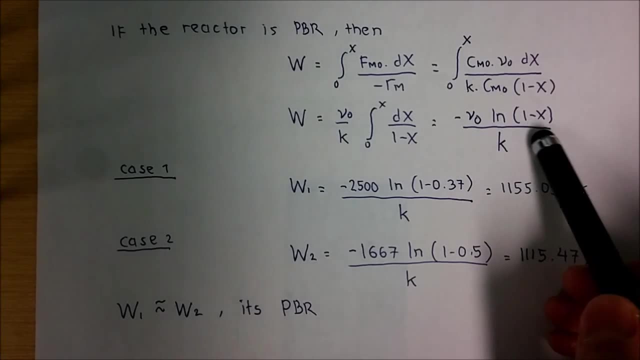 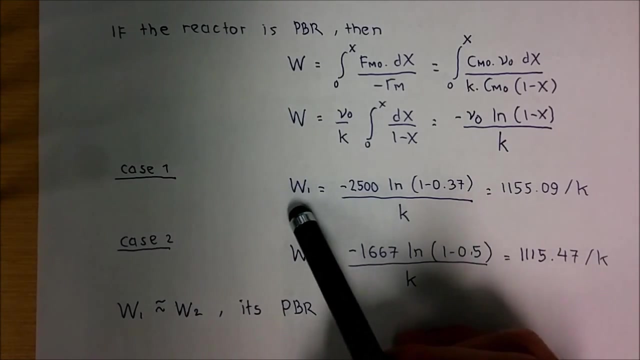 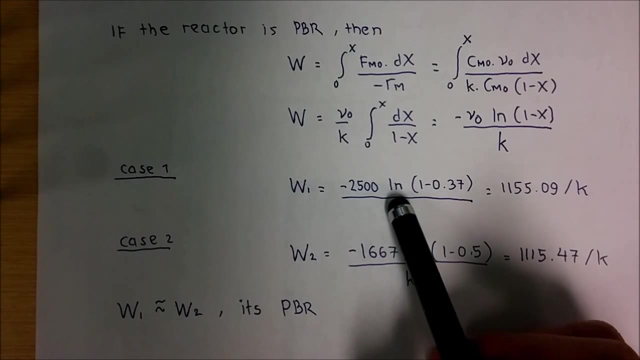 we're going to have. we're going to have w equal to minus v naught volumetric flow rate multiplied by logarithmic natural 1 minus conversion over k. and then, if we plug in the number for case 1, w is going to be equal to minus 2500, which is the volumetric flow rate multiplied by loan logarithmic. 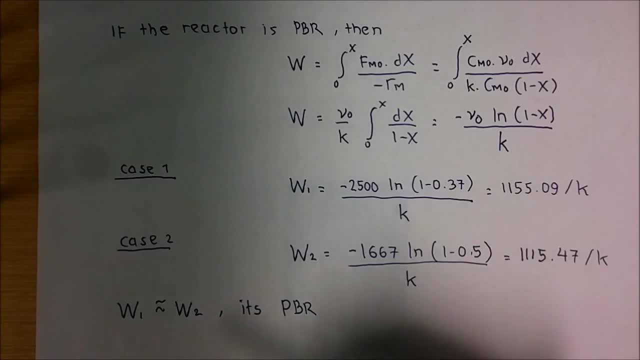 natural 1 minus 0.37, 1667 over k, we end up with the value of 1155.09 over k. and then for case 2, if we plug in the number, we're going to have w equal to minus 1667, ln. 1 minus 0.5 over k and we'll end up. 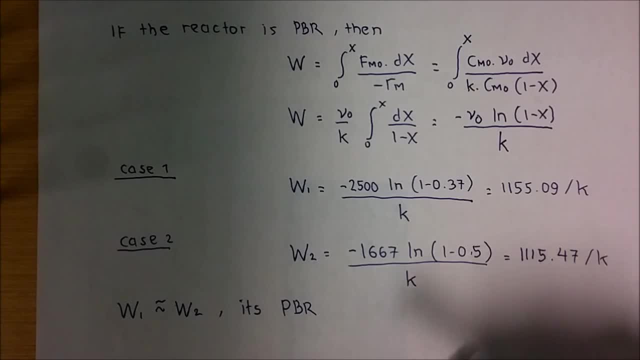 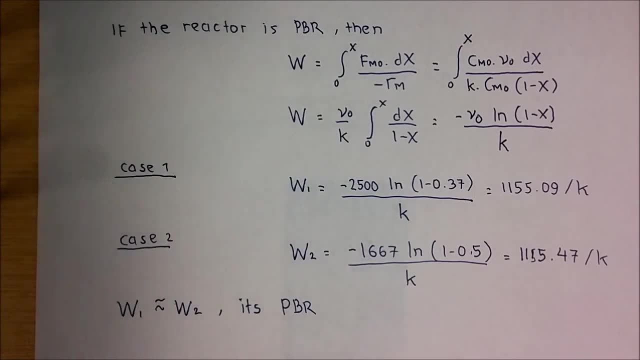 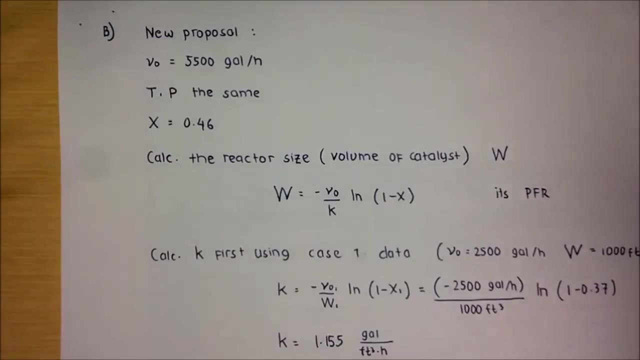 with the number very close, which is 1155.47 over k. so what? it means that w1 equal to w2 for the pbr case. so we conclude that the reactor is pbr reactor. now let's try to solve the part b of the question. 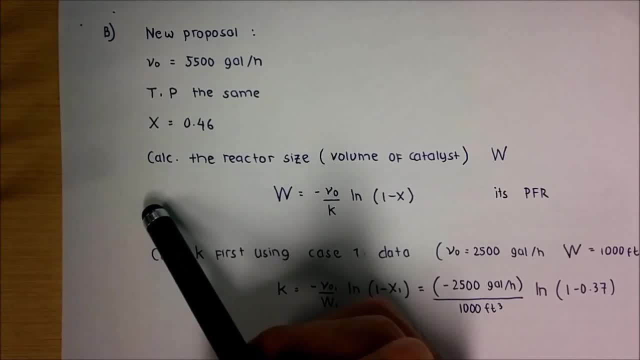 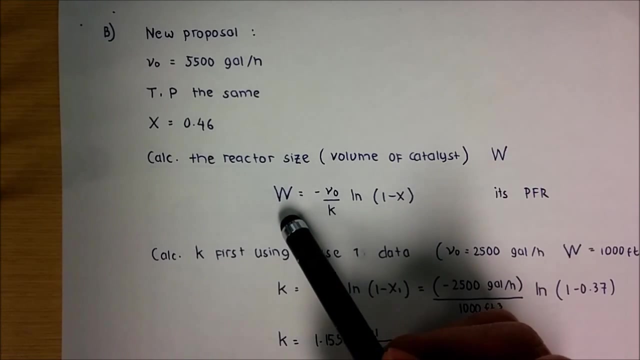 so in part b we need to find the reactor size for a new volumetric flow rate, which is 5500 gallon per hours, and a new conversion, which is 46 percent. so since we know that the reactor is pbr, then we can right away calculate the size or the volume of catalyst w. 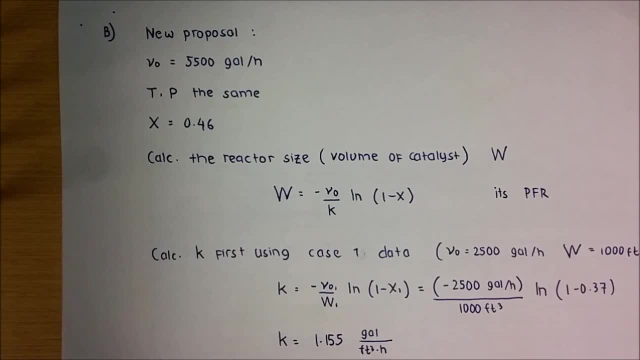 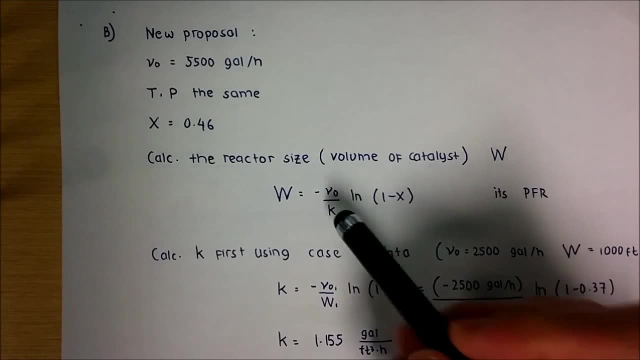 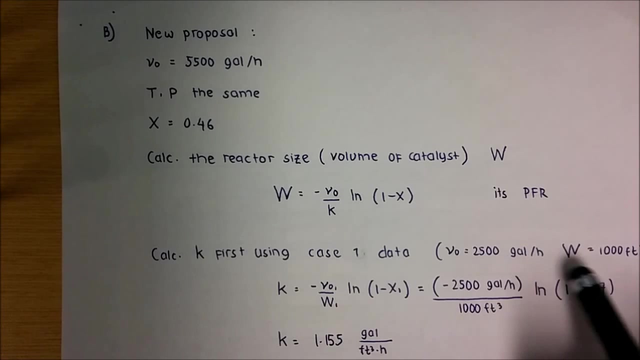 equal to minus 1667 over k, minus volumetric flow rate, over k multiplied by logarithmic natural 1 minus conversion. since we don't have the k-information, then we need to find out the k first, using the data from case 1, which is a volumetric flow rate of 2500 with the volume of catalyst about. 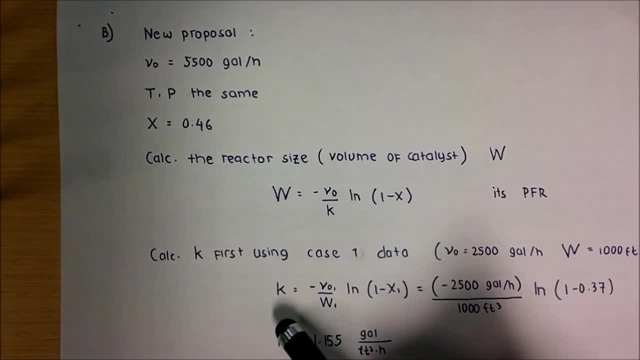 1000 feet cubic feet. okay, it's going to be equal to minus v knot over w剰 log ln. 1 minus x, which is rearranging from this equation. if we plug in the number, we end up with k equal to 1.155 gallon per feet cubic hour. 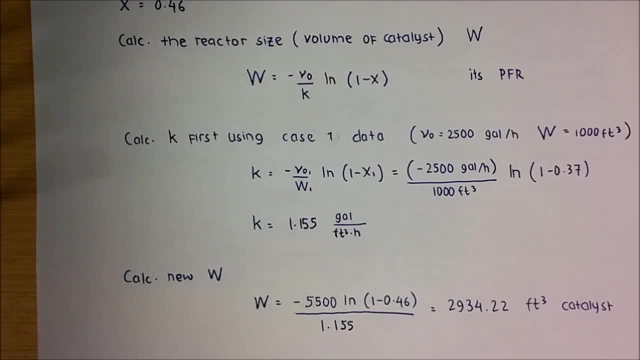 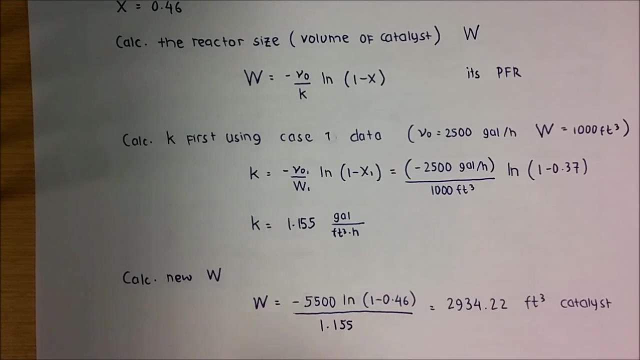 now we can easily calculate: the w, which is the new w, is going to be equal to 1.155 gallon per feet cubic hour, to be equal to minus 5500 logarithmic natural 1 minus 0.46 over k, which is 1.155.. We end up with 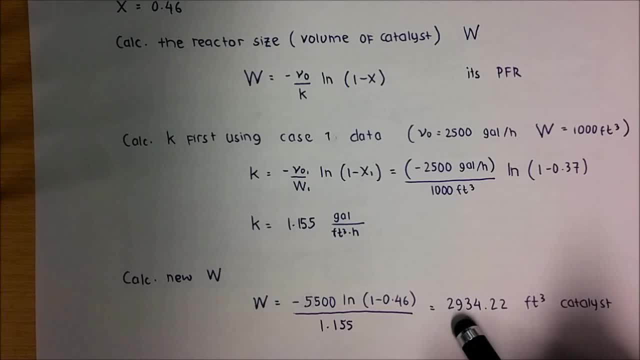 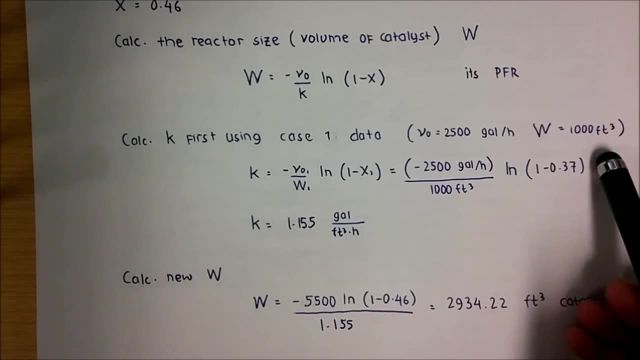 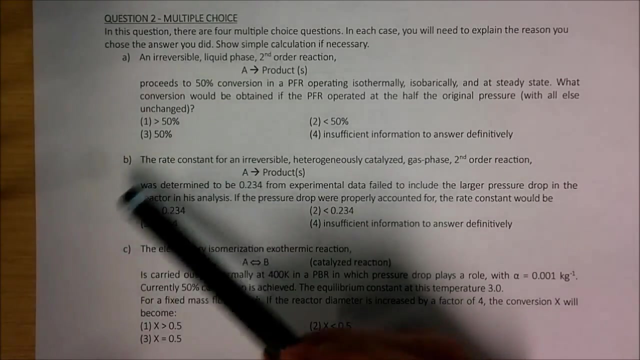 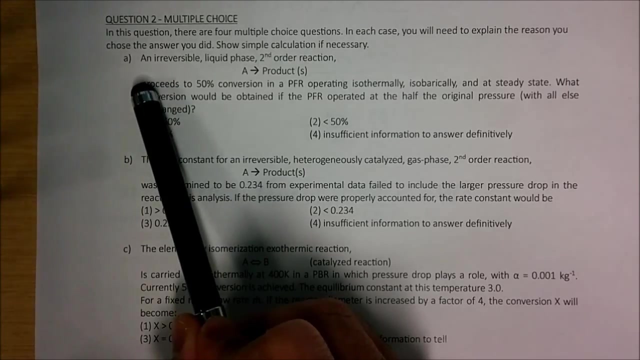 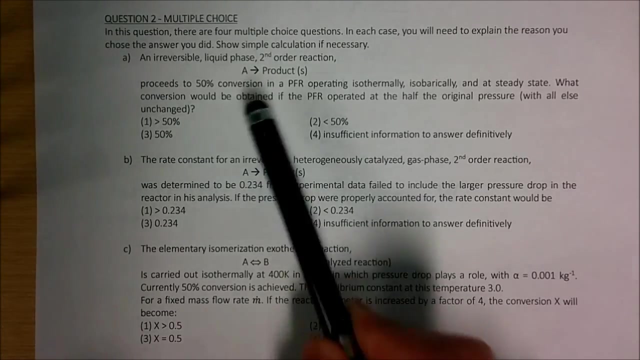 the volume of catalyst about 2934.22, which is much bigger than the volume of catalyst in case 1 and case 2.. So now let's move to the question 2, which is multiple choice question. So in part A we have, in a reversible liquid phase, second order reaction. The reaction is: A goes to product. 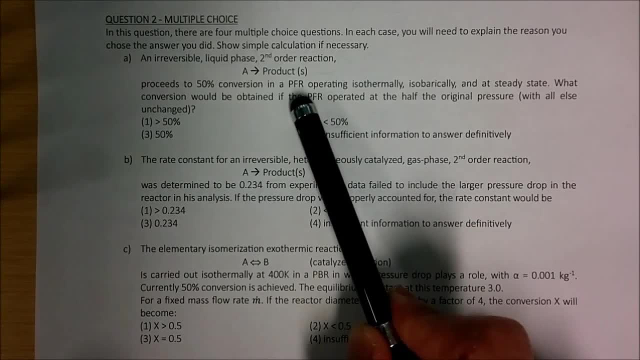 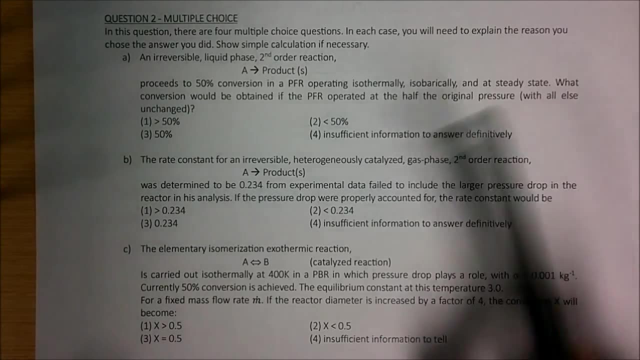 with 50% conversion in a PFR operating isothermally, isobarically and at the steady state. So the reaction is A goes to product with 50% conversion in a PFR operating isothermally, isobarically and at the steady state. The question is what conversion will be obtained. 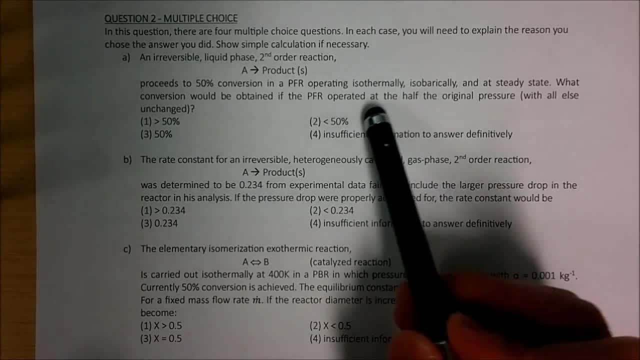 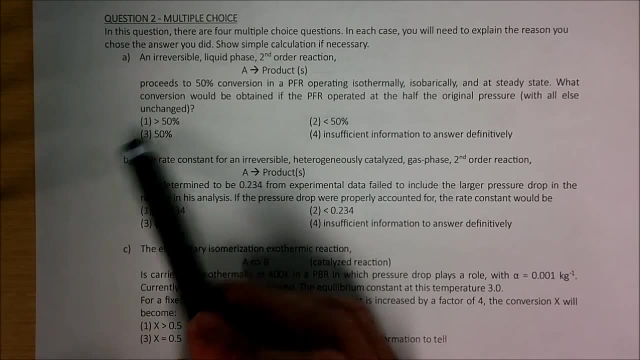 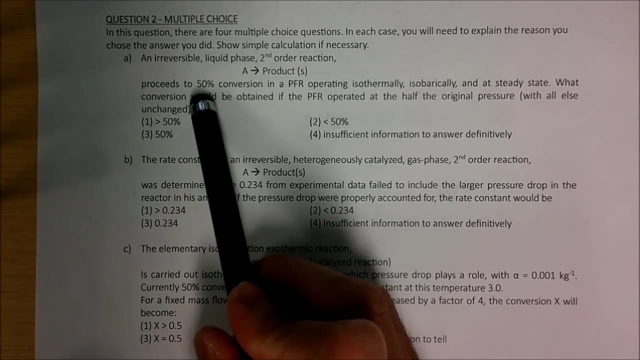 if the PFR operated at the health of the original pressure, with all else unchanged. So based on this question, we can easily see that the previous conversion, the original conversion, is 50% conversion. So the question is: what happened if we change the PFR operating at the steady state? 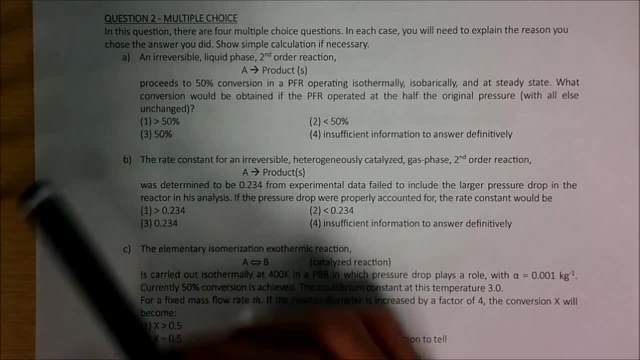 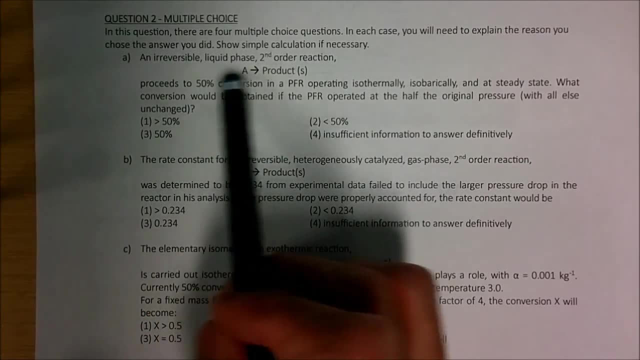 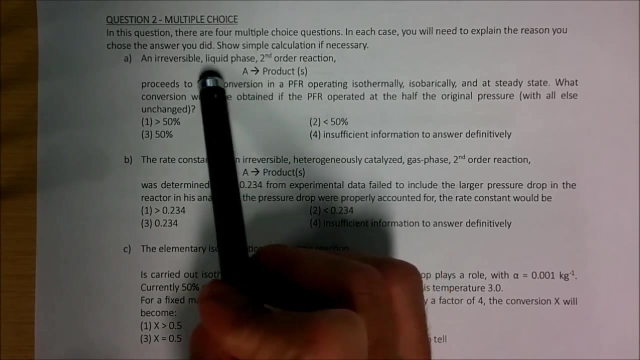 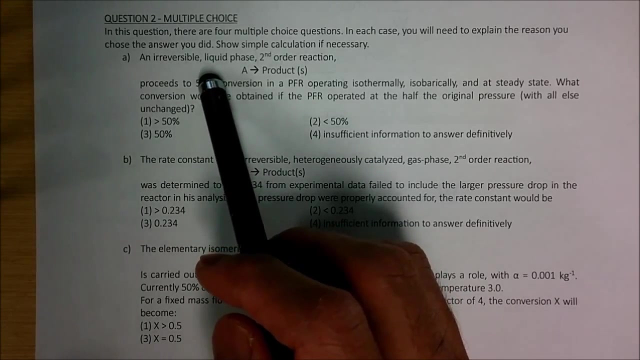 What we need to do is to analyze the information that we have in them For our first BUT in the first produce information, we see that the action is liquid phase and from what we have seen we learn that if we have liquid phase then, theyez мол, pressure effect is negligible. 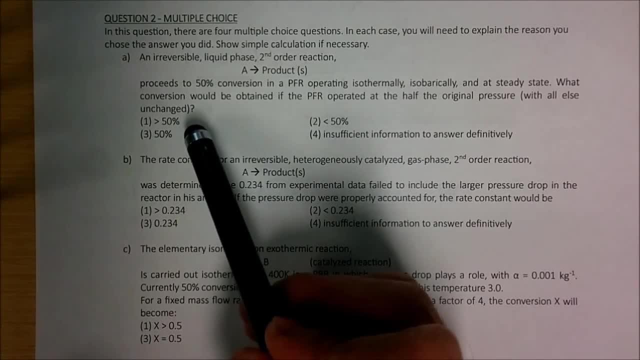 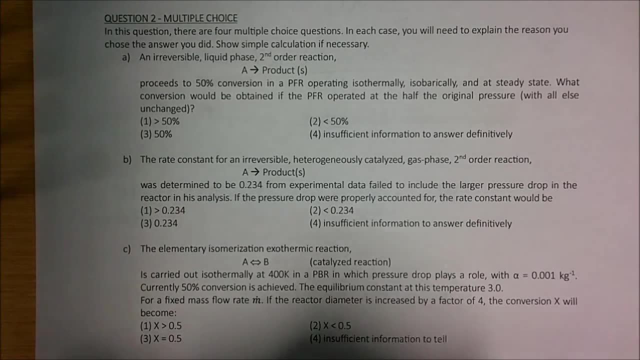 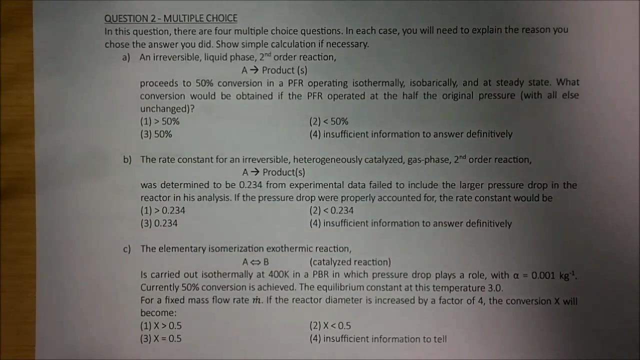 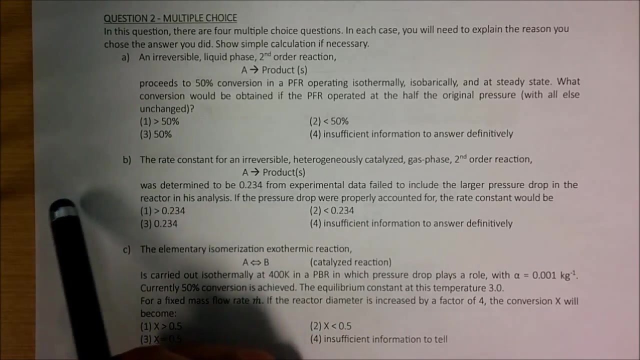 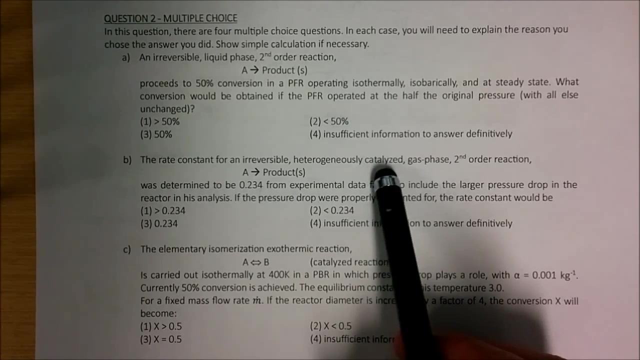 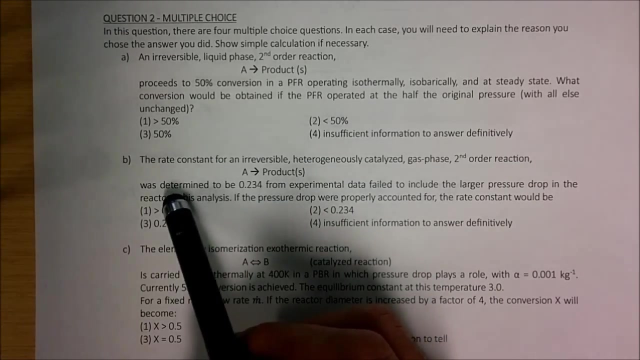 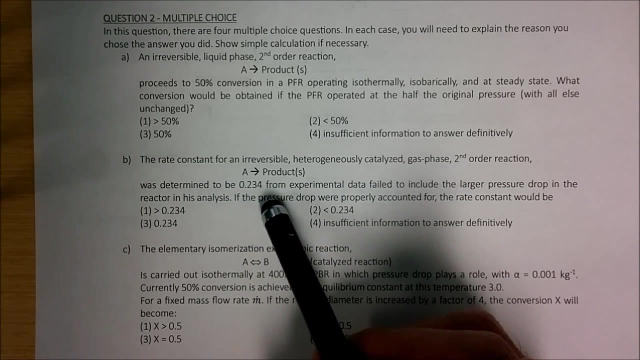 So we can say that if we run this reactor at different pressure, we're basically going to have the same conversion than the previous one, which is 50%. Now let's move to the part B of the question. In part B we have a reaction, irreversible heterogeneously catalyzed gaze phase second order reaction, and we also have information that the rate constant is 0.234, which is determined from experimental data. 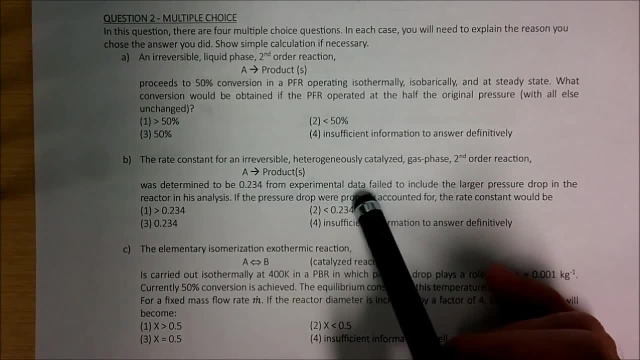 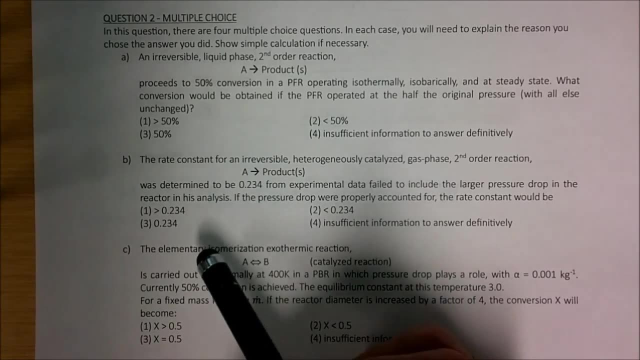 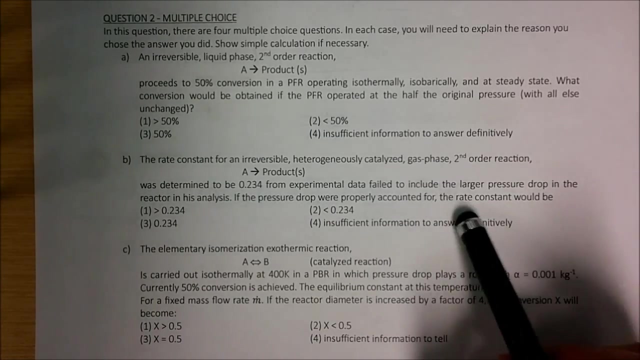 However, it says that the experimental data failed, So we're going to include the larger pressure drop in the reactor in his analysis. So if the pressure drop were properly accounted for, what's going to be the real rate constant? So in this question we need to find the correct K. 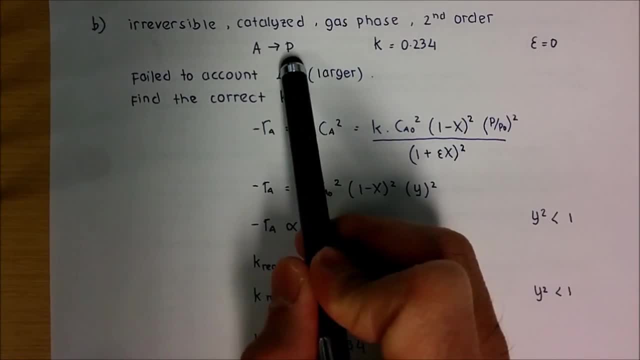 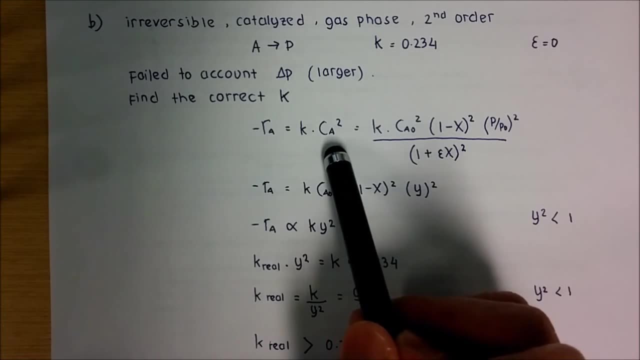 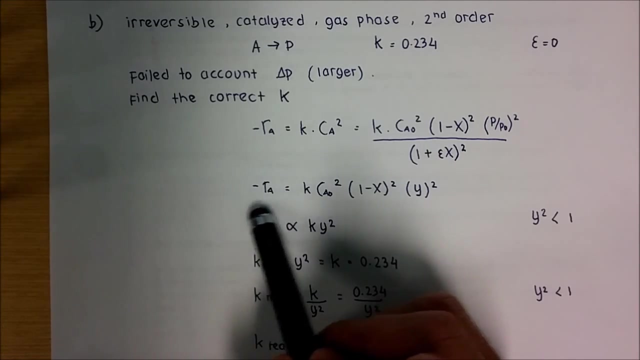 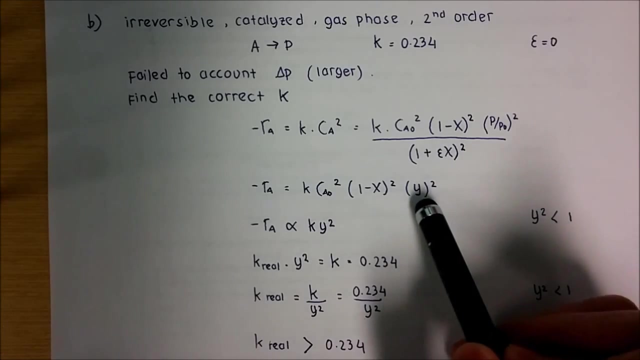 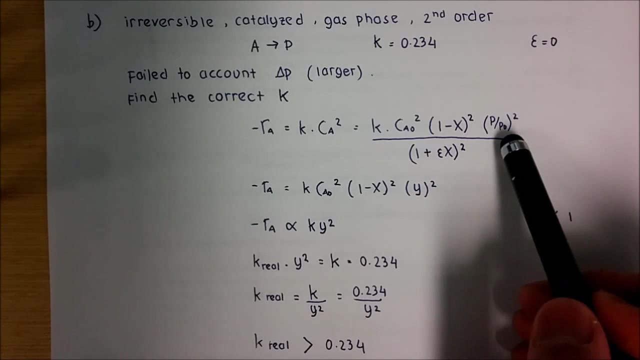 So if we have the reaction A goes to P, which is second order we're going to have the rate low is going to be equal to 0.. So if we have the reaction, B goes to K times C A squared, and if we're breaking it down based on stoichiometry, we end up having a rate low of K multiplied by C A naught squared, multiplied by 1, minus X squared multiplied by W, so multiplied by Y squared, where Y is actually the pressure change, P over P naught. 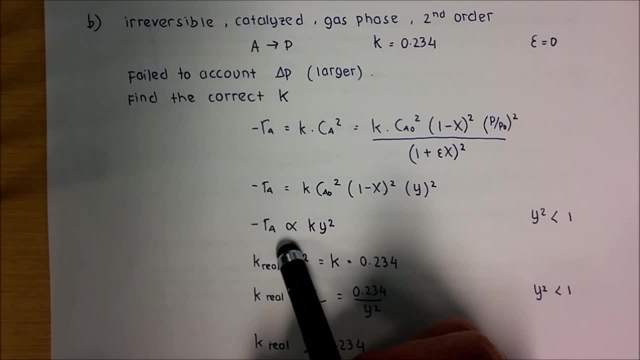 So we know that The rate low is proportional to K multiplied by Y squared, and we know, since the pressure change, Y squared is going to be less than 1.. So the K that we found previously, which is 0.24, 0.234, is actually the real rate constant multiplied by. 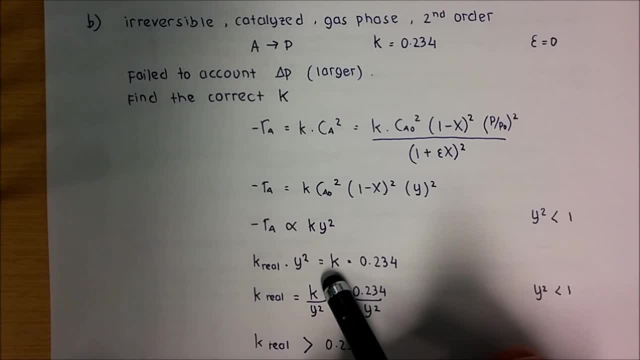 The pressure. So if we try to account the real, we have to calculate the real K, which is account for pressure change, and the K real is going to be equal to the K previously over Y squared. So if we plug in the number we're going to have 0.234 over Y squared. 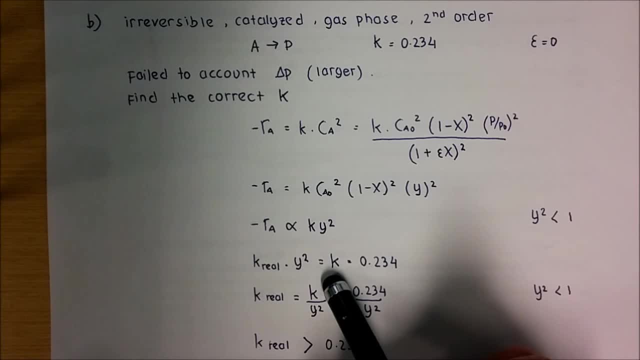 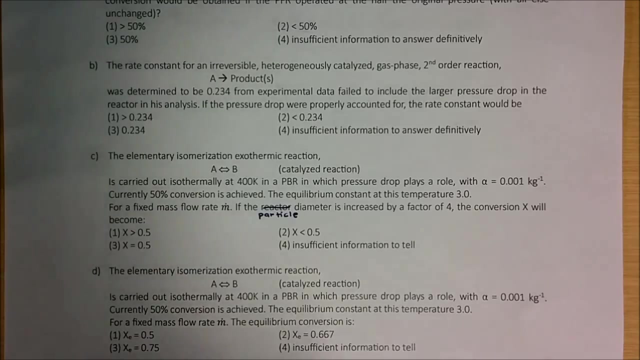 And since we know the Y squared is less than 1. Then the K real is going to be bigger than 0.234.. Now let's continue to the question, to part C. In this question we have elementary isomerization- exothermic reaction. 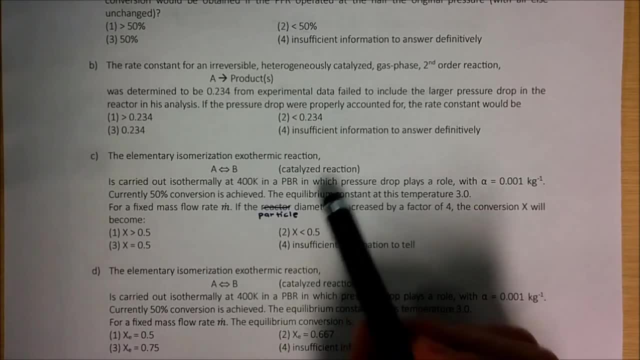 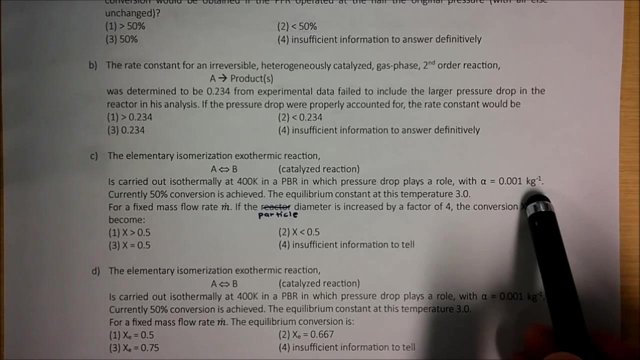 A goes to B and it's catalyzed reaction. It's carried out isothermally. It's 400 K in a PBR, which pressure drop plays a role, with alpha equal to 0.01 per kilogram, And we have 50% conversion. 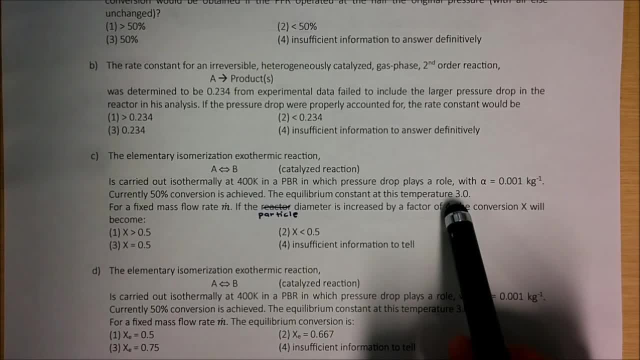 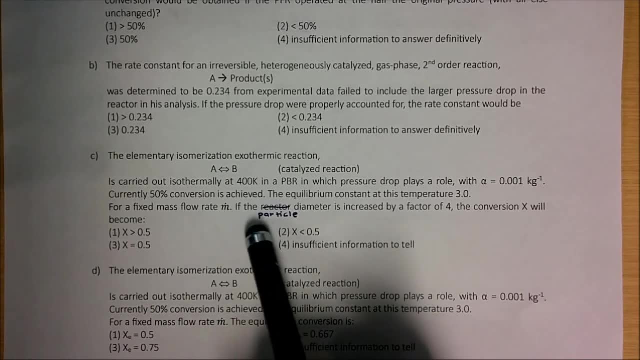 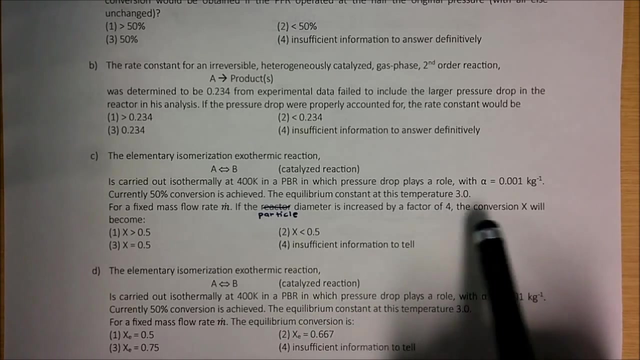 And we also have information that the equilibrium constant at this temperature is 3.0.. And if we know the mass flow rate, M, And if the particle diameter Is increased by a factor of 4,, what's going to be the new conversion? 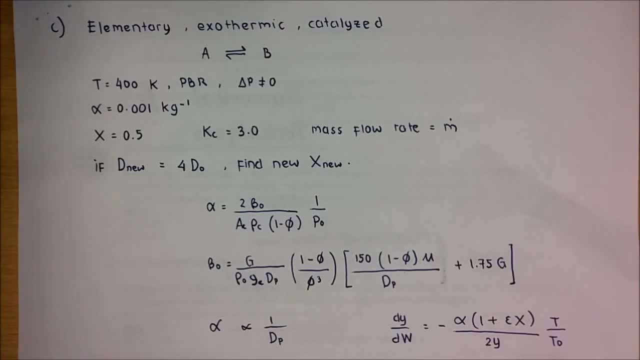 So we need to analyze the problem. Since we have the new particle diameter, which is 4 times the previous particle diameter, We need to find the formula that includes the particle diameter. So we know that. We know that alpha is actually related to beta and then a beta itself related to a particle diameter. 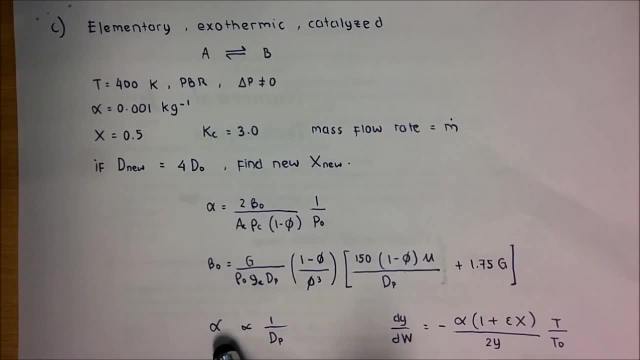 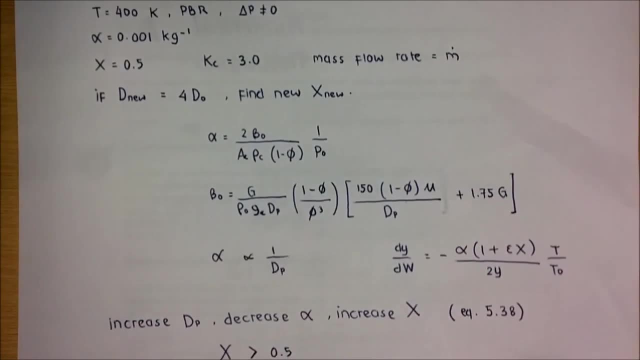 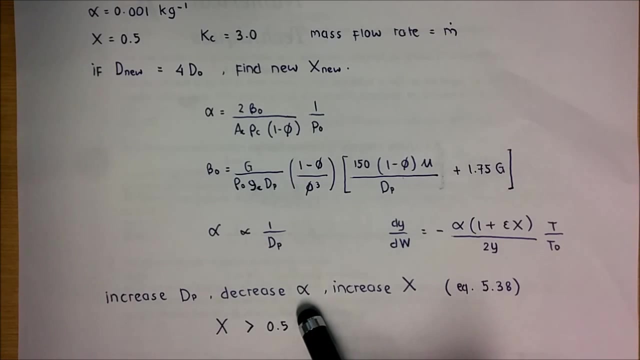 So what? it means? that from these two equation we can see that alpha is inversely proportional to particle diameter, And then we can conclude that if we increase particle diameter, it's going to decrease the alpha, And the other way around, it's going to increase the conversion. 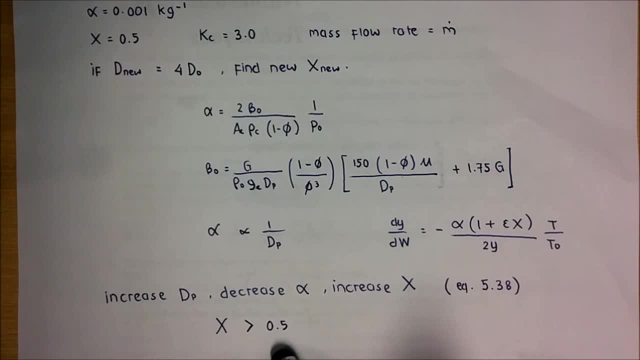 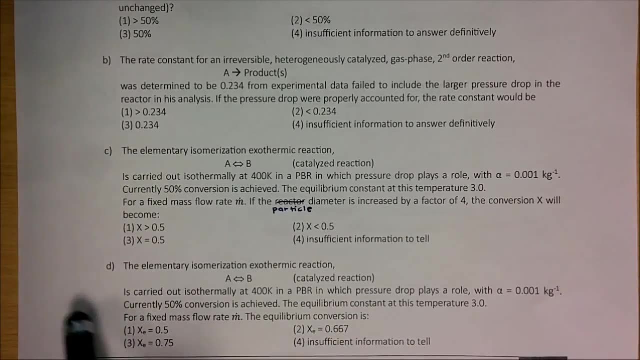 So we can answer that the new conversion is going to be bigger than 0.5.. So now let's go to the last part of the question, which is part D. We're going to have the elementary isomerization exothermic reaction. 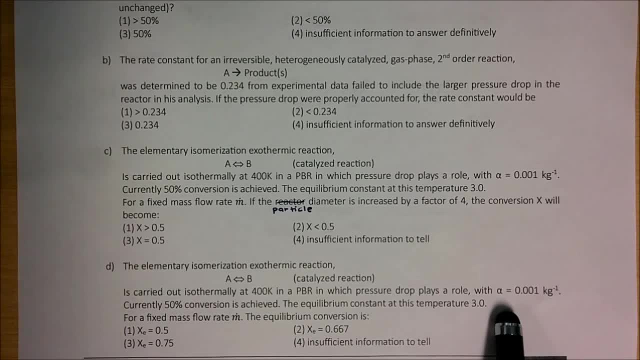 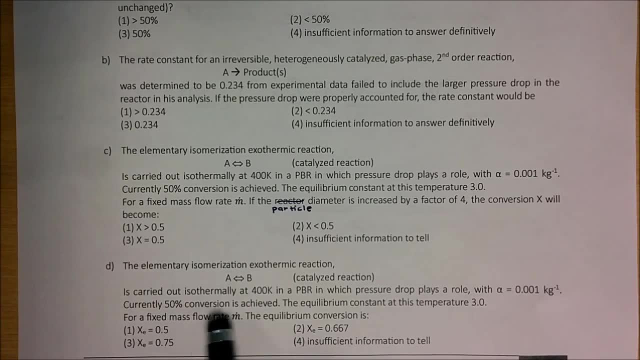 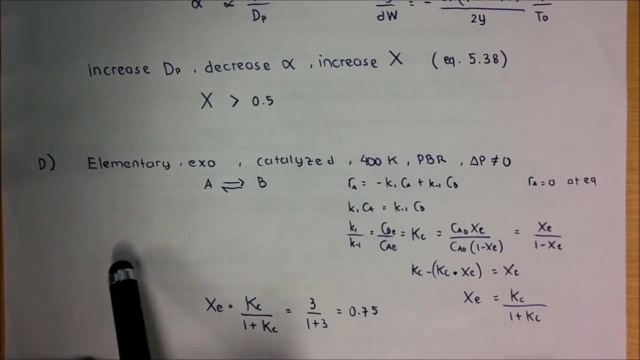 And then we have all data, exactly the same with the previous one. We have temperature, We have alpha 50% conversion, mass flow rate M, But the question is: what's going to be the equilibrium conversion? In order to solve this question, we need to derive the rate law of this reaction.